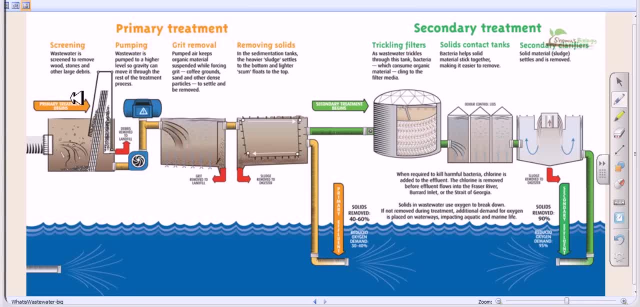 solid particles can. medium sized solid particles can also be separated. Now here we can see, in the primary treatment there are four different possible processes are given. One is the screening. Screening means simply: there are bar screeners like that we can just. there are comb like structure which can just. 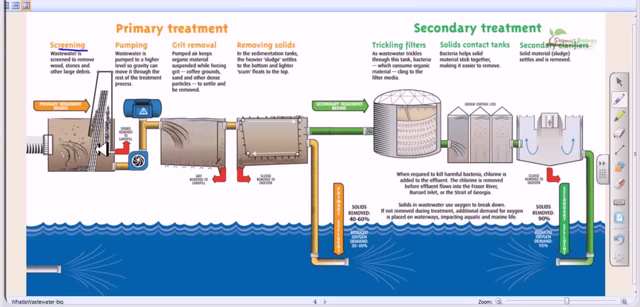 separate out the particle materials from this water. So there's a screen all the time, So it's getting up and down all the time, thus capturing all those huge materials out there and there are chambers. they just take those materials and put them onto the chambers and we take it and dump it. 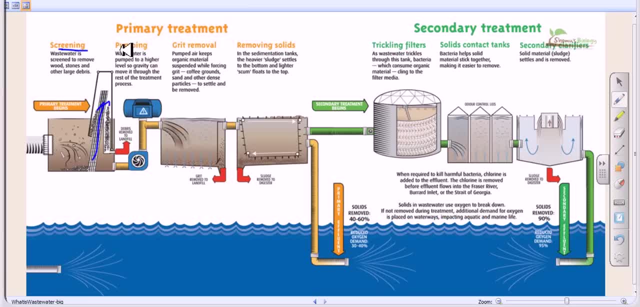 right. So this is the process. Now, in the second part, the pumping is there. the pumping is needed if you are having all the systems on the same ground or the same ground level. you're having this if you are dealing with this system in the in little. 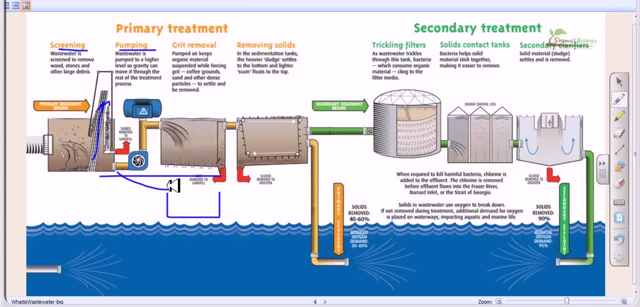 bit below level. in those cases gravitational force works very well. you don't need a pump. but in this case, in this, we have seen a pump. that means in this kind of wastewater treatment plant, all of this is all of the system, or all of the chambers are placed at the same ground level, right? 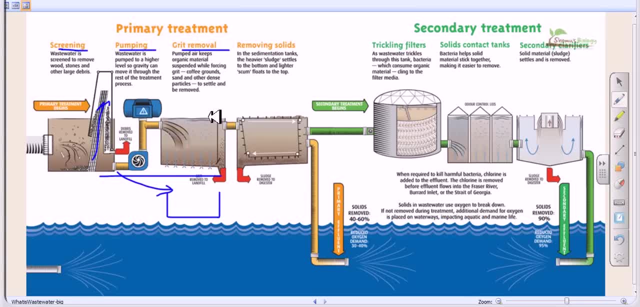 now the third part is a grid removal. now, in the grid removal process, grid means a very small, simple, uh, simple, or small stretches, or small, uh particles, uh, or particular particulate matters. now, the small particulate matters can be sand, can be soil- uh, you, big pieces of the sand and 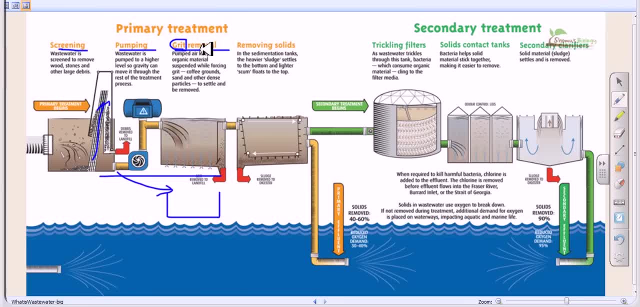 pebbles and all these things. these things will float. now in this grid removal process, we utilizes the physical method, like the gravitation, for to settle uh, this small particulate materials, down onto the vessel level. okay, and we can take up this uh material with us. 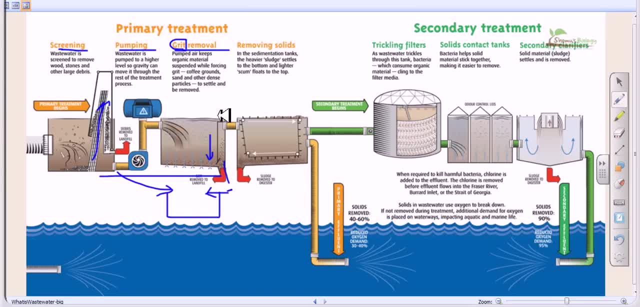 okay with us. so this is a process of great removal in this case. and the fourth thing is the removal of the solid. now, this removal of the solid is being taken utilizing the primary clarifier. i don't know whether it is showing or not, but primary clarifier is a very, very important part because in the 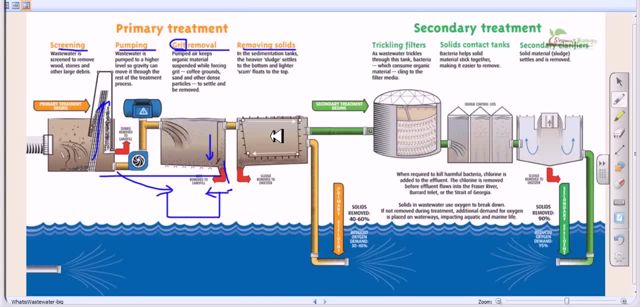 primary clarifier, the force or the speed of the water. the velocity of the water slows down almost to zero, so it's a pretty, pretty calm and cool area. the cool means not uh cold in temperature in this case. so in that case, what happens? as they are not having any velocity, so they just start to uh separate out. 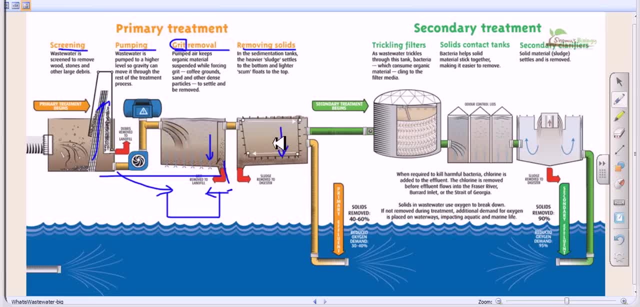 from the surface portion towards the bottom with the help of the gravitational force applied. now, and in this case, this primary clarifier also, there are uh regions, there are central part and there there is a scrum removal like this. now, what we call scum is is some floaty materials. 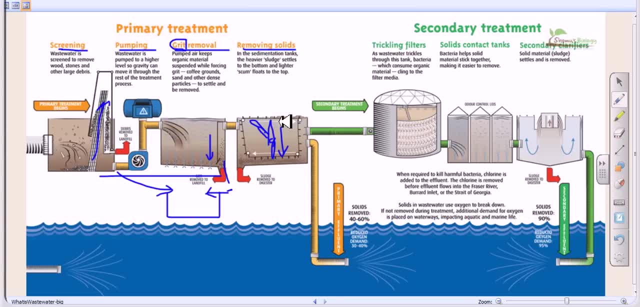 we start to float onto that upper layer of this uh primary clarifier. there are, there are some uh floating materials. we start to float onto that upper layer of this uh primary clarifier. there are, there are some regions, there are some portions or machinery process like that which just take all. 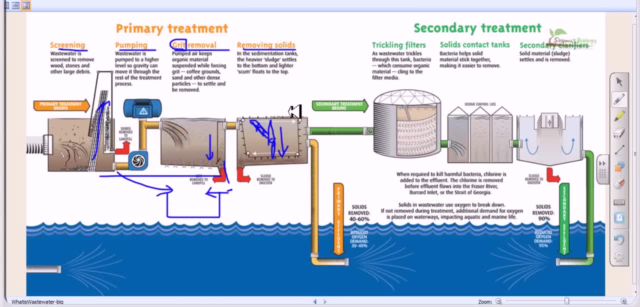 those things away and wash it into a particular area and put it into the dumpster. this is called the scum removal technique. now, scum is which is placed on the upper layer and grid is which is placed in the down layer. right now there is also a central, uh, bottom layer, center, bottom part, which 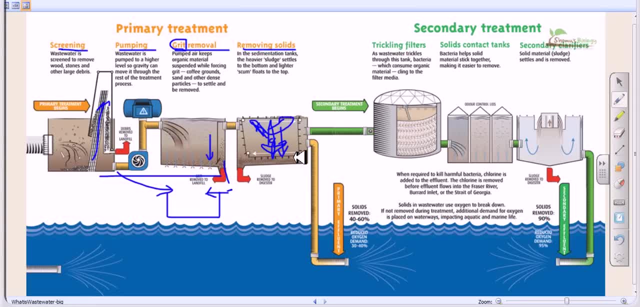 is also spinning, which is actually keeping on the flow, which is keeping the flow onto a particular area, which is actually helping those grid to settle down much easily now, as if these grids are settling down, as those small particles are settling down, that they can be taken up as sludge. 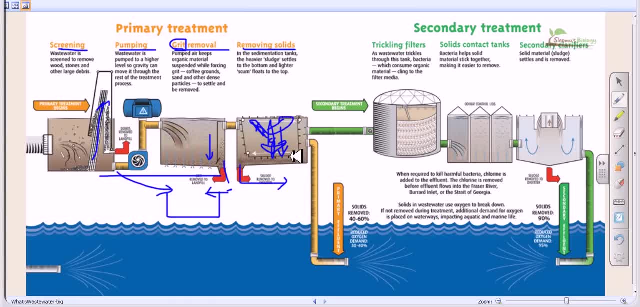 so we call them sludge because they are also nutrient rich. those nutrient can be nitrogenous nutrient and phosphorus nutrient. so they take up this nutrient and we utilize it in this, in the sludge treatment procedures, which are totally different from this liquid treatment. now right, 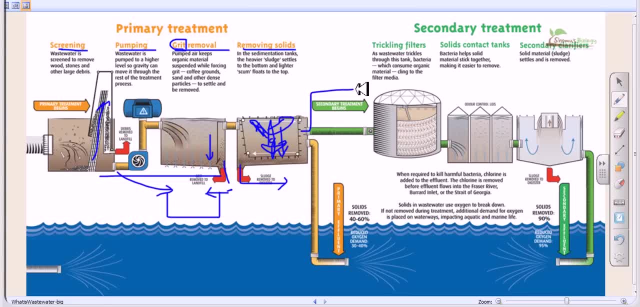 after this primary clarifier, it will go this: this water or effluent will go to the secondary clarifier for the biological treatment. because in primary treatment, all of the techniques we are utilizing our physical means or having physical technique procedures. now, in all these cases, what we are looking at, whether we are we are utilizing sedimentation, will coefficient. we. 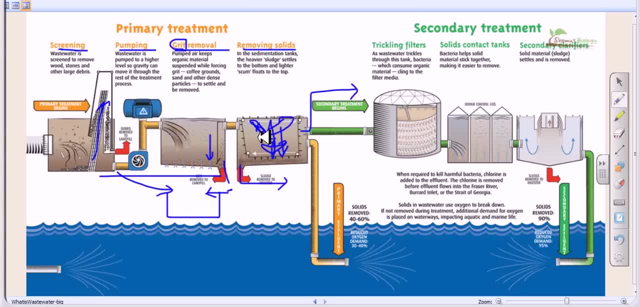 utilizing the gravitational force and we utilizing the velocity and utilizing all those scar, all the scum removal techniques, utilizing this screener techniques. all of them are the physical means, methods of separating the solid particles out of the liquid particles. so this is the basic goal of the primary treatment and then in the secondary treatment we will deal with the organic materials. 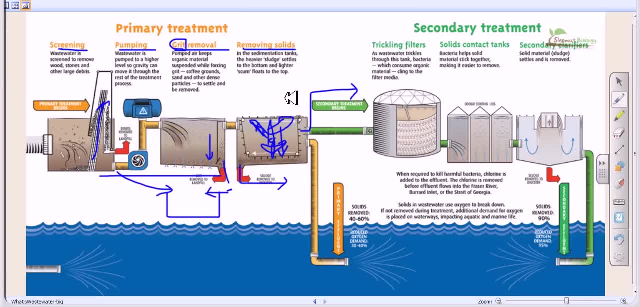 or organic waste, which are present in this wastewater, which is present in the figuratively fairly high amount. now, we can do this utilizing the biological weapons, like, like microorganisms, like bacteria, protozoans, and all this. we put them onto the nutrient, away onto the wastewater. they 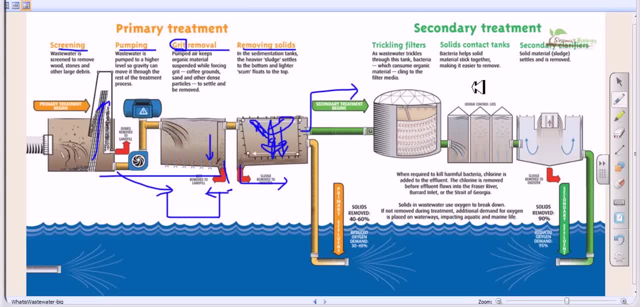 uptake the nutrient from the wastewater- all this waste materials like nitrogenous waste or phosphorus weight- as their nutrient. they they will take from the water and, as a result, water will be purified and it will be ready for taking it on to the third and final layer of this wastewater treatment, which 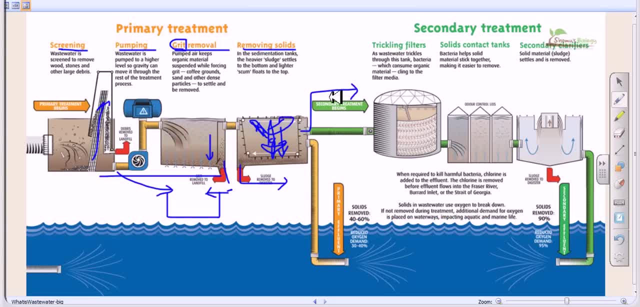 is the chemical treatment. so this is how it, the whole process, is being done. as you can see, in all these cases, effluent will be taken and the solid will be take for the sludge, sludge processing. okay, so this is a process of primary treatment. now, the right after the 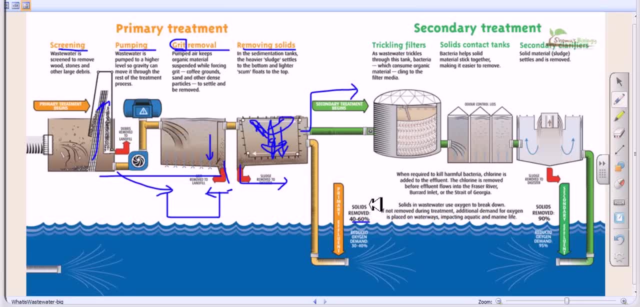 primary treatment, 40 to 60 percent of the solids are removed, as you can see in this case. so the primary treatment is basically deal with the solid removal. now in in those kind of wastewater treatment plant where we have both type of physical treatment facility, like the preliminary treatment, as well as 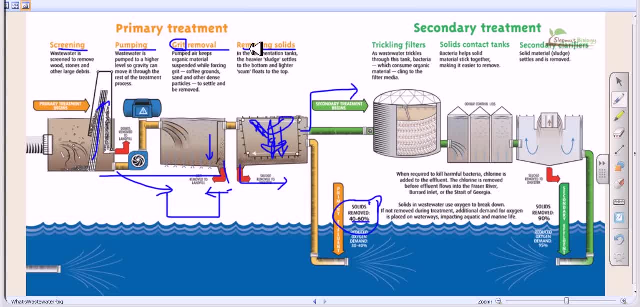 the primary treatment. right after the primary treatment almost 70 to 80 percent solid materials are separated or are being removed- in those cases right, and also in this case, 30 to 40 percent of the dissolved oxygen or reduction of the biological oxygen demand is 30 to 40 percent right after the primary treatment. but 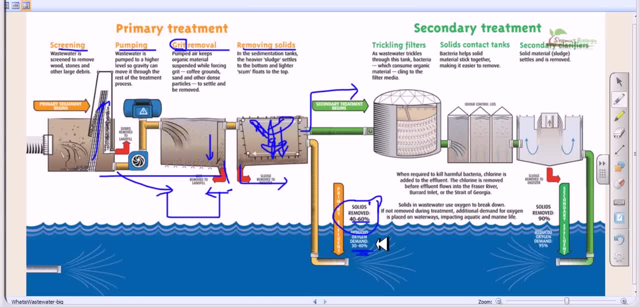 that is not too much effective because still it contains the phosphorus waste and the another waste which are toxic. now that's why we need to go through the second round, because organic wastes are dangerous. it will be harmful, so utilizes bacteria to kill those organic waste. and finally, right after, 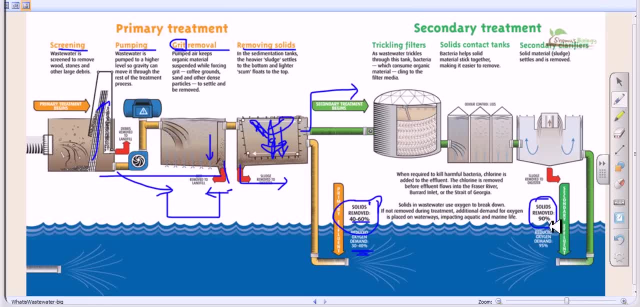 the secondary treatment. you can see 90 percent of the solids are solids are removed and BOD- up to 95 percent are removed right. so this is the process of primary treatment and I hope it will help you, thank you.